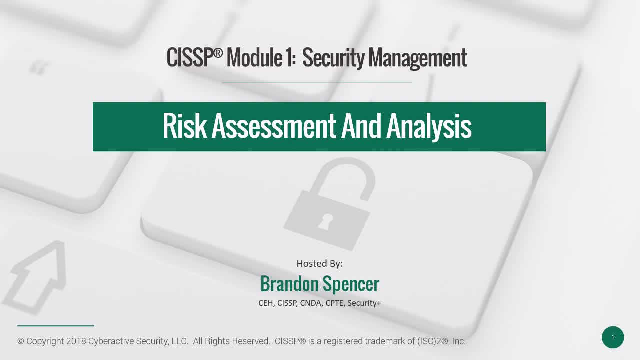 coaching call that I did recently for our complete CISSP students, And it's all about risk assessment and analysis. Now, if you're not already subscribed, make sure that you smash that subscribe button and click that notification bell, So you'll be the first to know when a new video comes out. And, if you like, 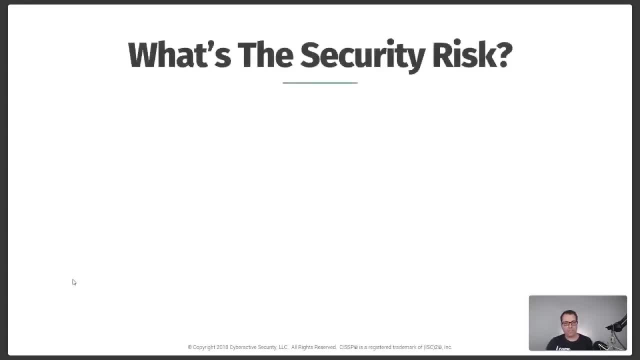 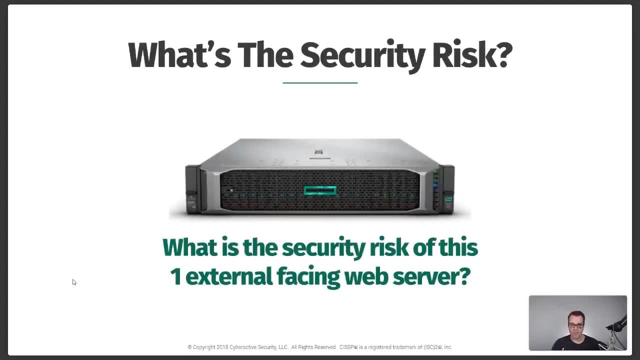 what you see here. please give it a thumbs up. So let's bust into risk assessments. Okay, this is a web server In the chat box. I need you to help me out here. What is the security risk of deploying this web server to an external facing interface? You're going to deploy this. 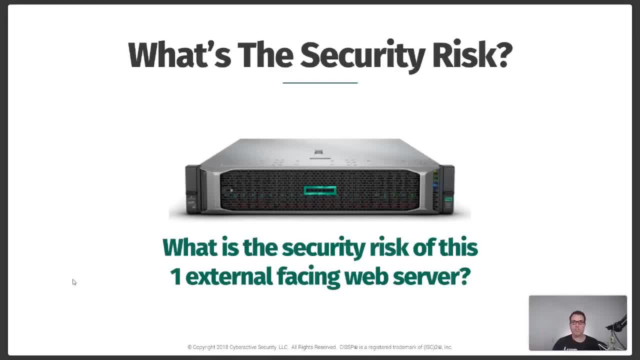 server and people from the internet are going to connect to it. Tell me in the chat box what are some of the risks of this. So that's why it's a workshop. We're going to do some work. I hope the chat box isn't lagging. It seems like it is All right, So I'll just keep going, just in case the 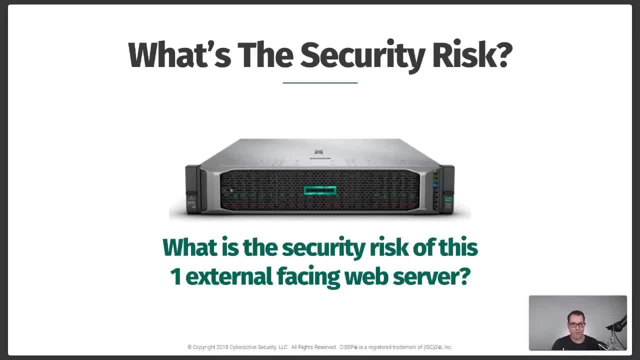 chat box is dork. Yeah, So you got somebody saying a DDoS attack, distributed denial of service- Yep, Okay. What else? Okay, Cross-site scripting. DDoS attacks- Right, What else? SQL injection attacks- There you go. 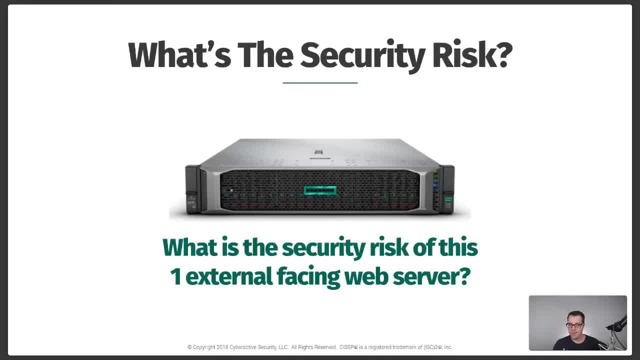 Next, What else we got? These are good, These are great. Keep them coming. Andrew needs a firewall. Okay, DDoS, SQL injection, risk of exploit, leak of information- Yeah, Little lag, but you guys are bringing it in Good deal. Leak of information, Cool. 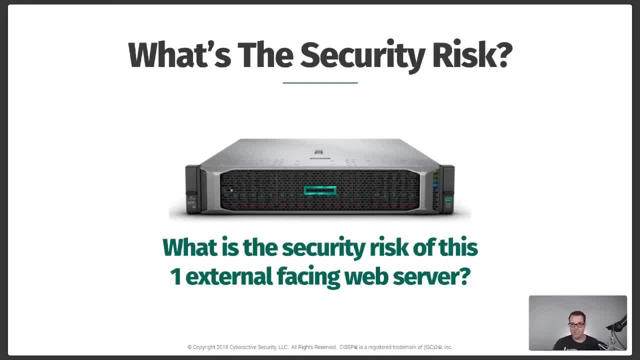 So here is where the fun comes in. Yeah, Information spills. Yeah, totally. So here's where the fun comes in. I'm just talking one web server with an external facing interface. I didn't mention that I had a gateway server, a proxy server. There's a VPN that goes to it. 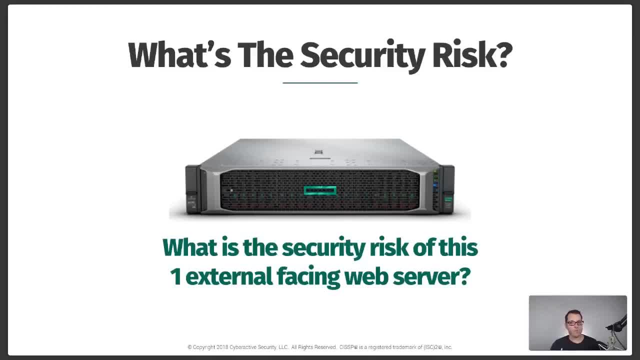 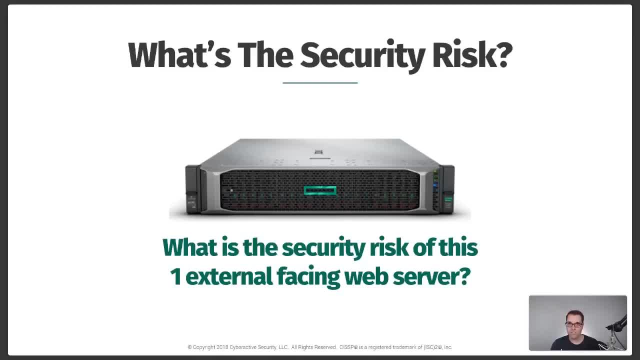 the risk. You drop a firewall. Once you put a firewall in place, it changes the risk, doesn't it? If this thing was just external facing and just sitting out into an open zone where anyone from the internet can come in, I don't think that server would last five minutes. It would be gone. 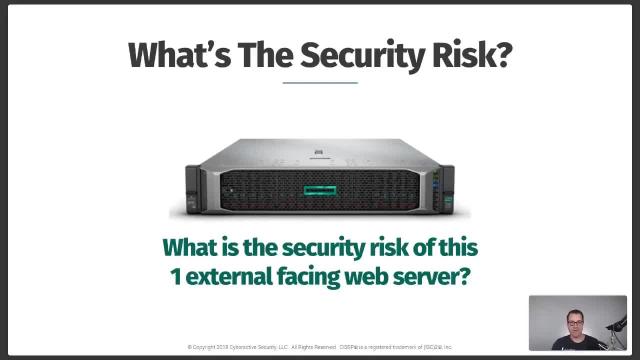 right, Somebody would just eat that server alive. But do you see how, all of a sudden, you start thinking of all the things that can happen? right, You've got ransomware attacks, You've got leak of information, You've got risk of exploits, DDoS, SQL injection, all that different stuff. 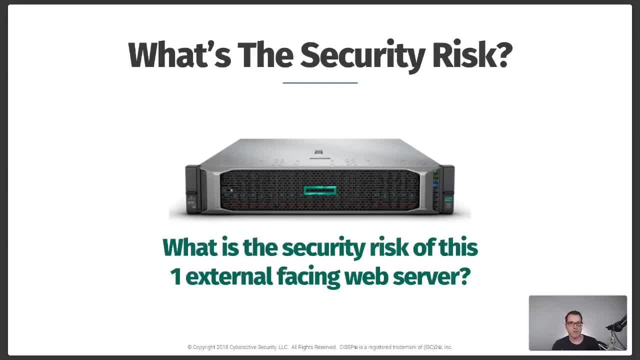 But here's the funny part: A SQL injection won't affect the server. We're talking to app. at that point right, Whatever web app is running, If we have a GUI, if we have just a web app that's facing and interfaces with, 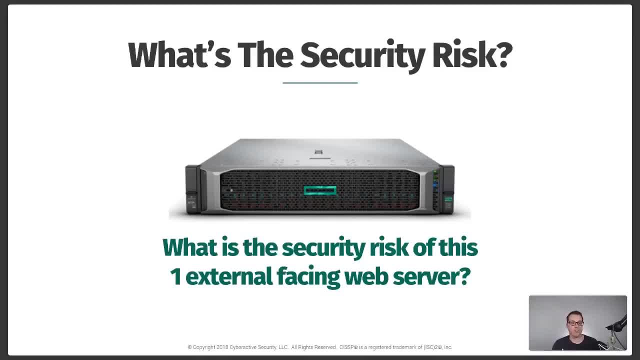 a database, there's your SQL injection. But what if this is just an external web server that's hosting image files? right Now we're not worried about SQL injection because we don't have a database in the backend. We've got everything stored right there, right. So now you see how. 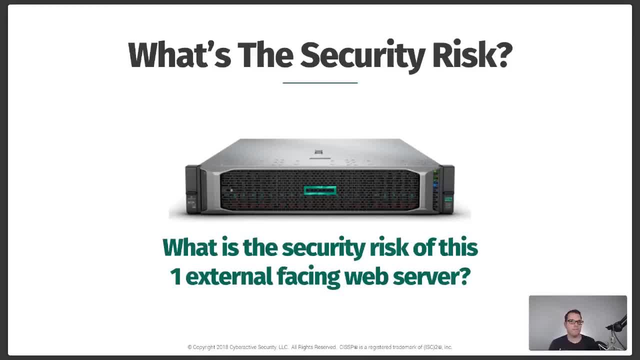 all this starts working. If you don't understand this piece of it, how are you going to be effective at doing any kind of work? You're going to have to do a lot of work. You're going to have to do a lot of. 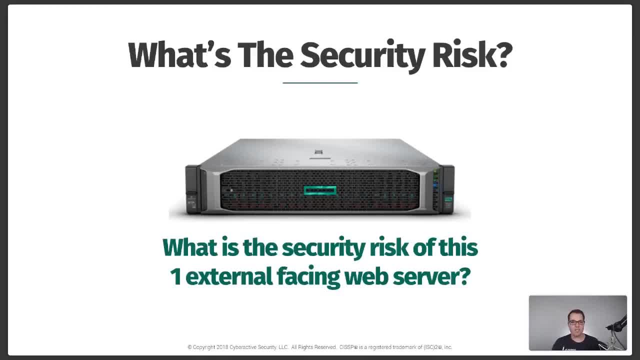 security assessment, right. So if you don't get these pieces in place and start thinking, okay, yeah, this web server can sit there, but then what? And I like where everyone's going, You guys have your head in the right space, right? Cross-site scripting: You got DDoS attacks, I mean. 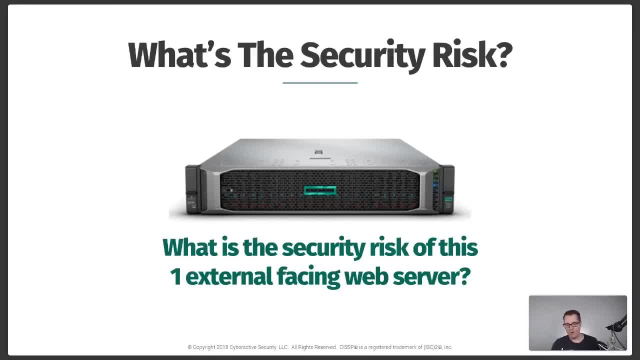 somebody would be like: oh, you could do a lateral movement and do this. Whatever man, whatever you guys want to throw in there, The idea is, what is the main thing that we are? what is the main thing we are chartered to protect in cybersecurity? What is our crown jewel? 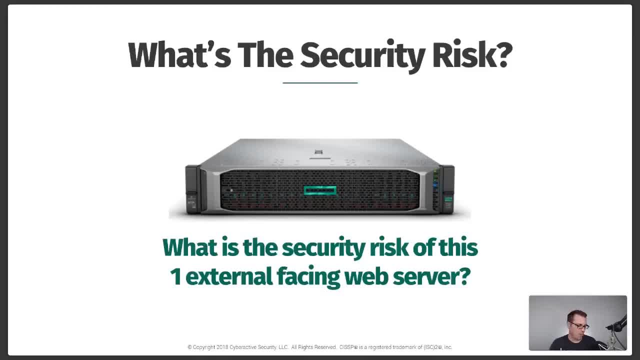 What's the one thing we need to worry about more than anything else? Tell me in the chat box What's the one thing in security we need to worry about the most. This is always a great question because I get a ton of answers and I love it. 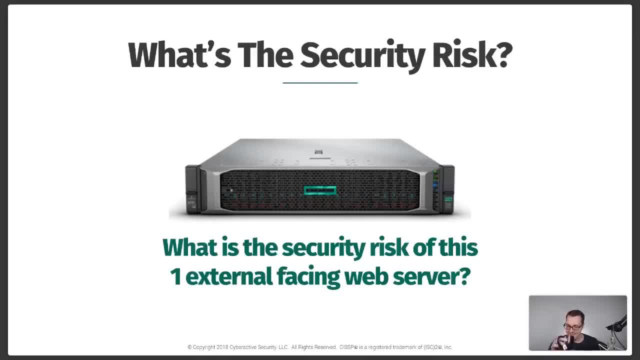 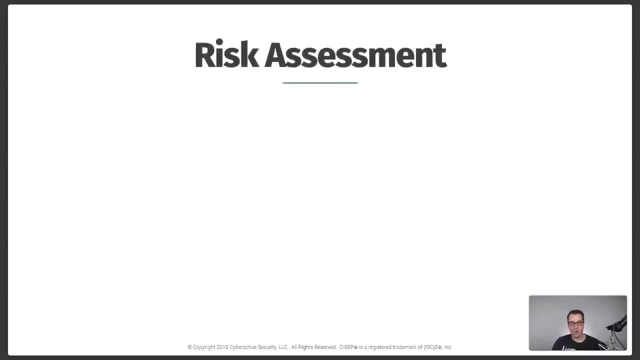 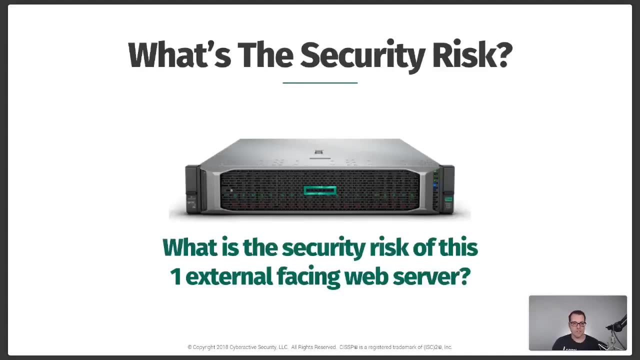 Andrew, don't cheat man. You know the answer. Cool, Everyone has the correct answer. Your data is your crown jewel. So tell me this. Let's say we go back. Let's say this is an external facing web server. Okay, Roy. 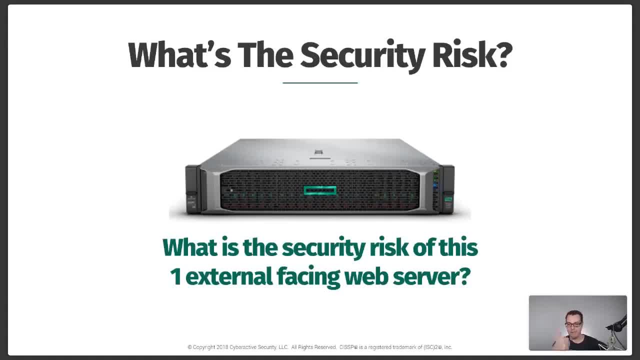 you're in my CISSP class, brother. That's a perfect answer. Good man, I like the answer. So let me change the paradigm on you. This web server is external facing, has no data. Now, what's your risk? Has no data, What's the risk? Who cares about a web server? Who cares? We can. 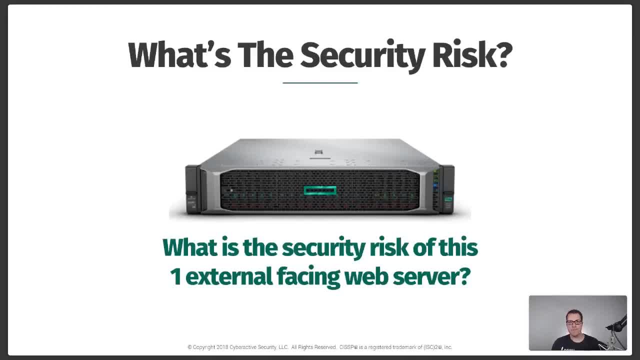 rebuild that Like that right. Who cares about that? But see, we get so caught up in the hardware part of it Why? Because it's sexy, It's awesome. I mean, who doesn't love running tools and seeing results and? 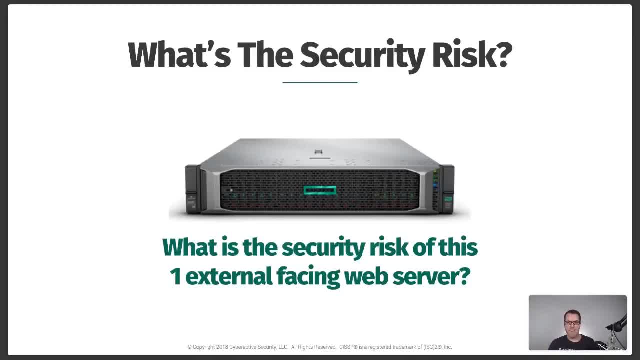 banging on a web app and watching it crash and going ha, ha, ha ha ha. That's fun. That's fun to do. Your web app sucks, dude. You need to go back and work on this. That's fun, But. 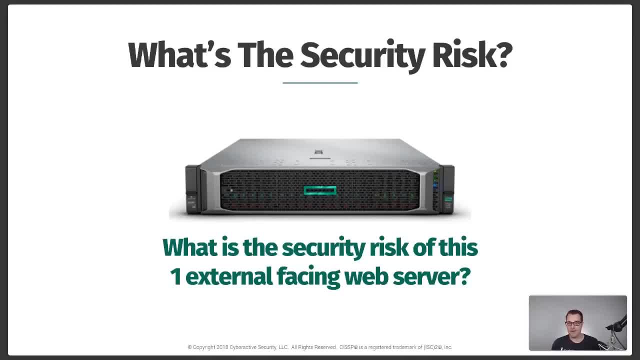 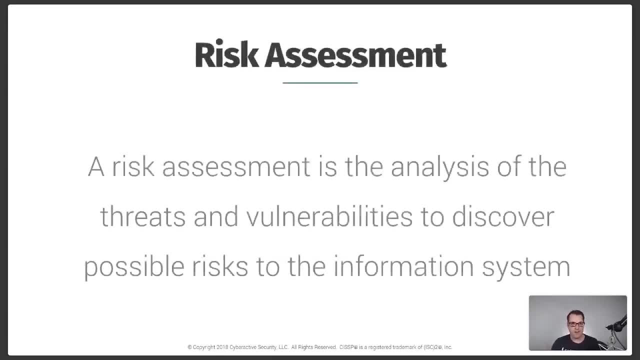 this is the real thing right here. This is what we're all after: The data. You are after the data, protecting the data. So if this server has no data, it doesn't matter, right? So when we're running a risk assessment, 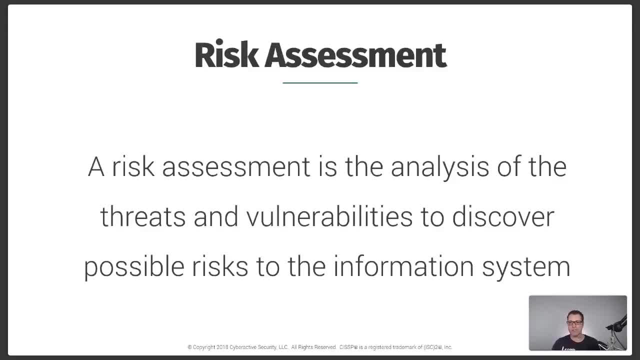 we need to analyze the threats and vulnerabilities against that particular system, And you just did that live in the chat box. You're analyzing what are the threats. Threats are DDoS, cross-site scripting, SQL injection. Maybe you've got ransomware, I heard right. Well, that could be. 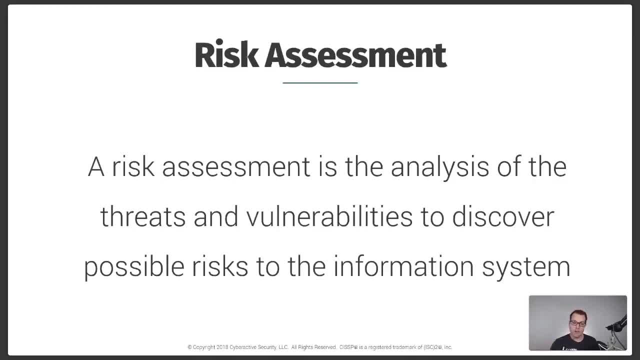 a little bit different depending on what kind of operating system is running on the web server. But the thing is, it's all subject to all those different things. So now we have to go back and we have to analyze what those are right. 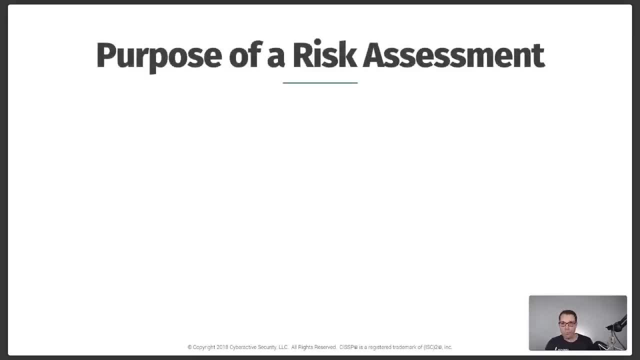 What are those things And what is the probability of that happening? So the whole purpose is to identify those organizational assets. We have to know what assets we are supposed to be protecting, What assets have what kind of data on them. That is the most important thing. 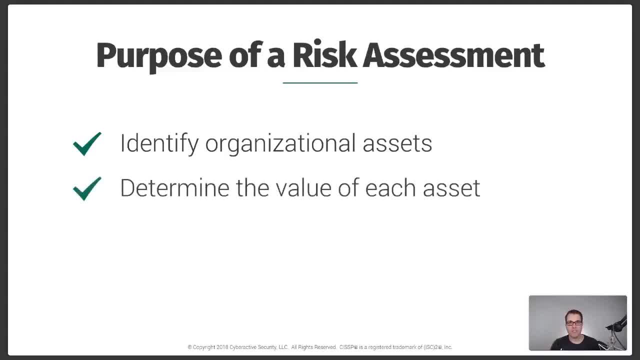 Then we have to look at the value of each of those assets. So if we have a web server that we're going to put out on the internet- don't know why we're going to do that, but we are for the sake of conversation- How much is that web server worth- And it's not just the 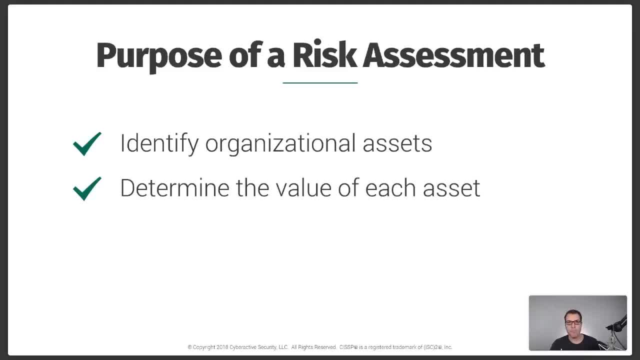 the web server. How much are you going to pay a system administrator to rebuild it? How much are you going to pay us to go do an incident response right? So now we have to go triage what happened. How much are they going to pay us to do that? That all gets added into that value. How much? 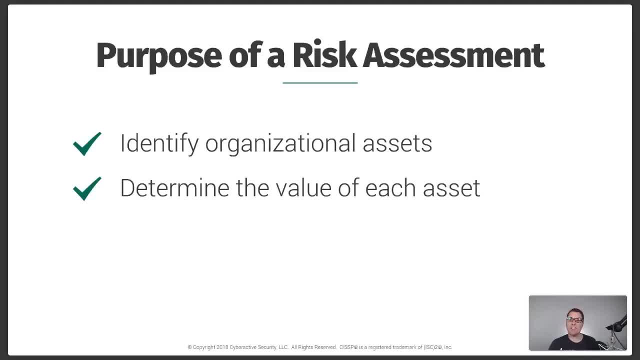 is that data worth? If that data on there gets spilled and it gets leaked out to the outside world, how valuable is that data? What is it going to do to the reputation of the company? Now, if we're having that conversation, you really didn't do a risk assessment, because if you're, 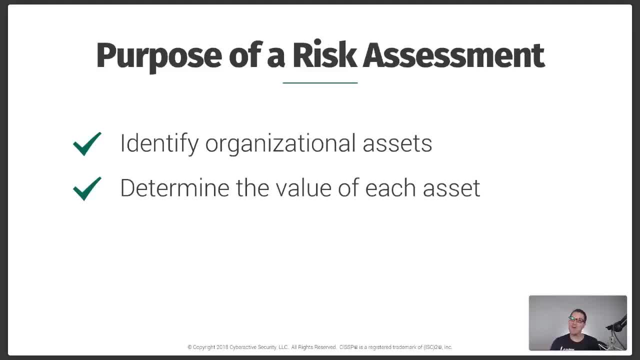 going to put sensitive data on external facing web server. we got bigger problems, Like we need to have a conference right So, and then we need to assess the threats and vulnerabilities. We need to know who's going to come in from that outside interface and get to that data right. Those are. 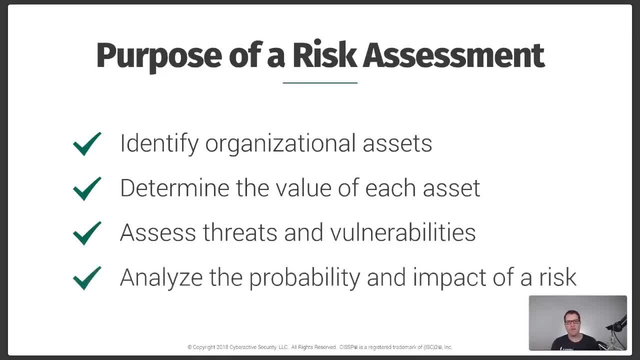 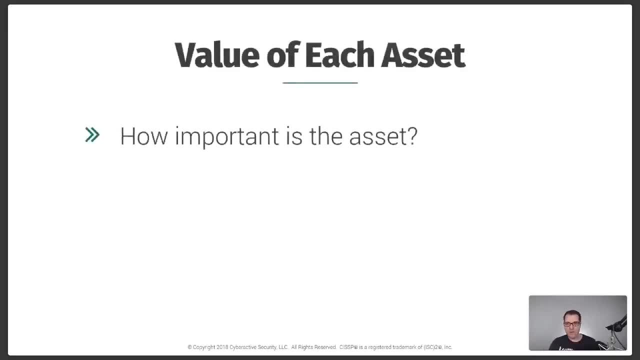 the most important things that we're doing as part of this risk assessment, And then we put it all together and then we take a look at the probability and then we impact. you know that risk, Okay, So the value of each of the assets it comes into how important is the asset If the asset is a risk, it's a risk. If it's a risk, it's a risk If it's a risk. it's a risk, If it's a risk. if the asset were to be compromised, how is it going to affect the organization? How much is it? 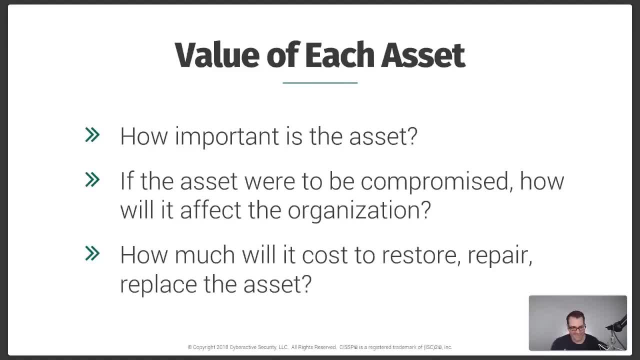 going to cost to restore and repair. I know this stuff off the top of my head. How about that? I wrote this slide right. That's what's most important. What? how important is this asset? Is that if that web server doesn't have any data, then who cares? Let it go right, We'll just 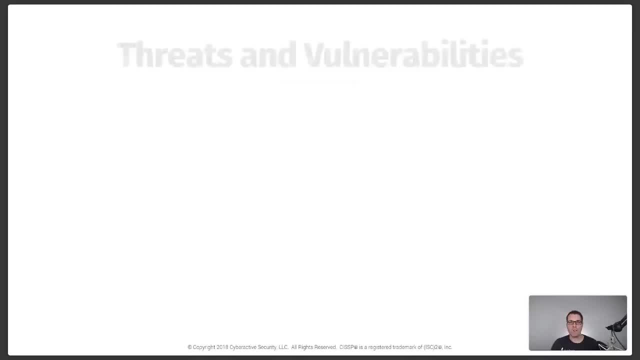 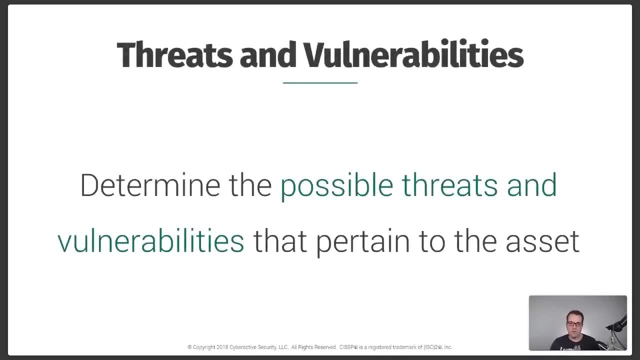 rebuild it No big deal. But if they have asset gets compromised, then how much is it worth to the company? So threats and vulnerabilities: are we need to look at the at what is actually going to be the true threat and vulnerability to that particular asset? 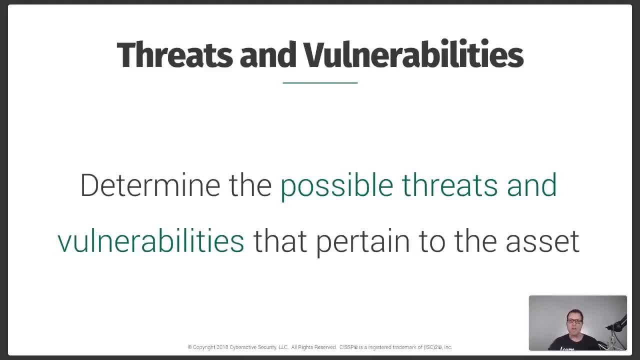 Asset that we're performing, the assessment on that we're looking at. It's not to the entire enterprise, It's just to that asset And that's what you can do in your head If you're going to do an enterprise risk assessment. that's a, that's a. that's a lot of work. That is not easy. 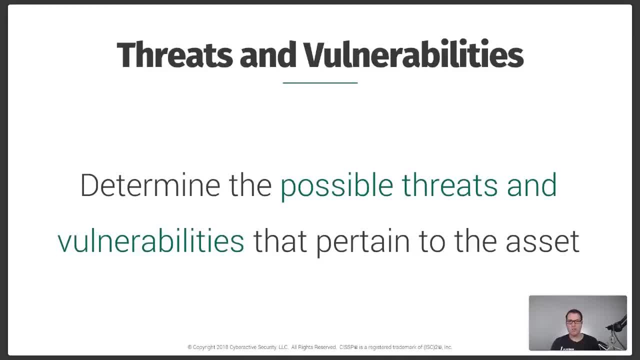 That's not something you can do on the fly, but for one asset, sure, You could definitely do something and get close And and then at that point maybe even take it back to a piece of paper and say, okay, now let's piece of paper. How old school am I? open up a word doc or a. 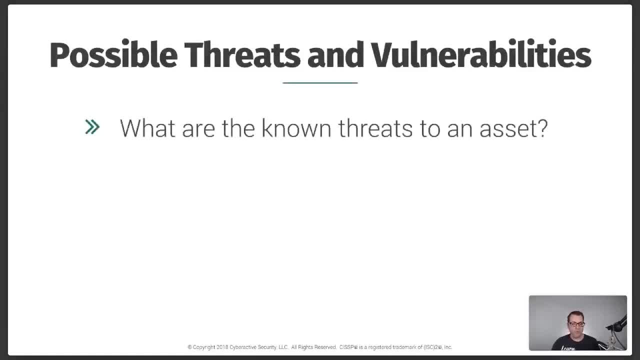 assessment tools. Okay, So possible threats and vulnerabilities: we already talked about a little of them, but we want to know what kind of threats are really going to attack that asset. What are the known threats to that asset? Because we do know that web servers don't have the same. 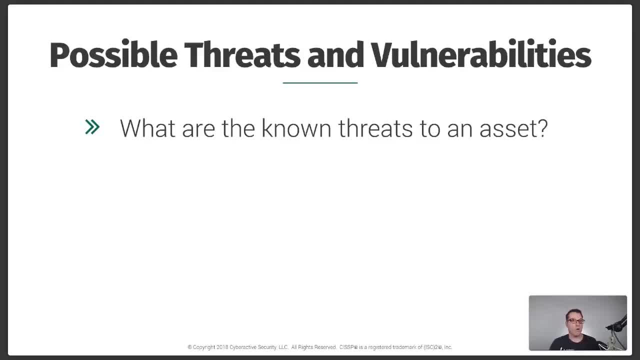 vulnerabilities, as say, a data server or a workstation, a mobile device, right, A network device like a router, switch, proxy, firewall, whatever it is right. Not all threats are the same and not all vulnerabilities are the same, Like we just talked about with the SQL injection, right, If you're not running a web app on that web. 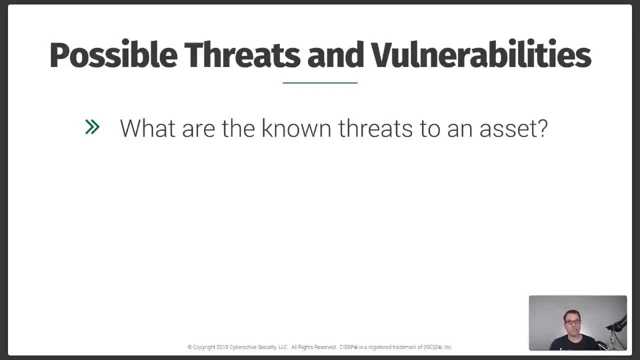 server, you can't inject anything. You can do an LDAP injection against it- Maybe try to break in that way- but you're not going to do a SQL injection against it If it doesn't have a SQL database on the backend right. So now we can check that one off the box, Okay, So also you. 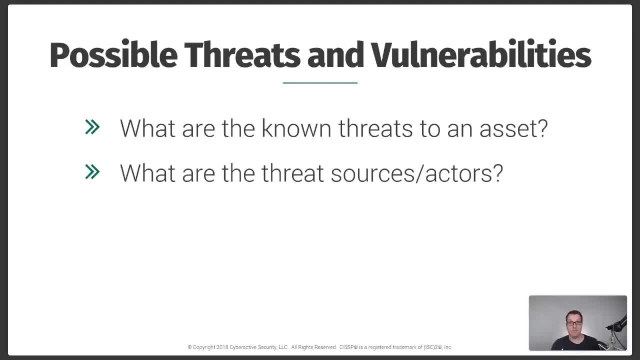 want to look at. what are your sources and actors? So if it's facing the internet, it's everyone. you're going to have a ton of people coming after that thing. And again, what are the known vulnerabilities in the firmware, in the operating system? 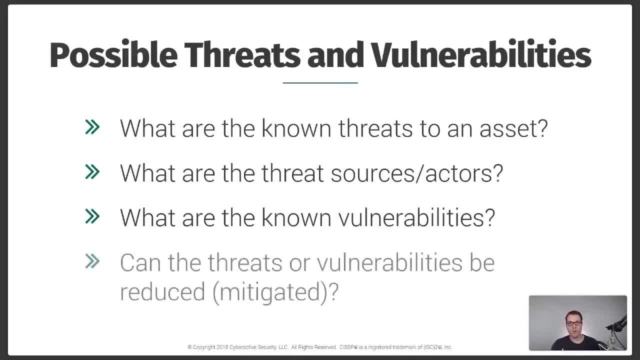 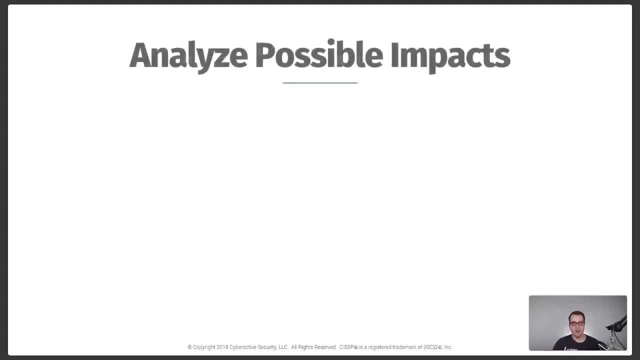 In the applications that we're running. what are the known vulnerabilities And also can those be mitigated? So now we're stepping into risk management a little bit. Okay, So, analyzing those, you want to take a look at what can go wrong, right When you have stuff plucked in. 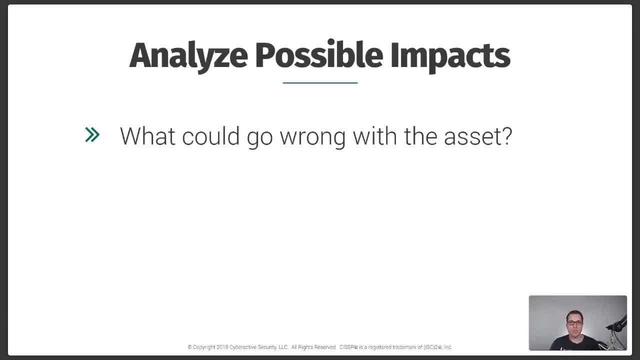 what can go wrong with this asset? So when you're installing a server tomorrow at work or, you know, thinking about installing a server somewhere, if you're doing that, you have to think what can go wrong here. Maybe you're going to install that web server and it's. 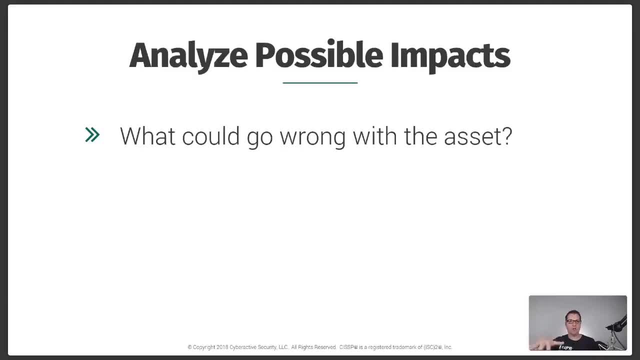 going to run in parallel. right Run together. So you already have a web server running. You're going to put another one and it's going to run, you know, at the same time, And maybe you're just going to do a cut over because maybe we're upgrading, or something like that. What can go? 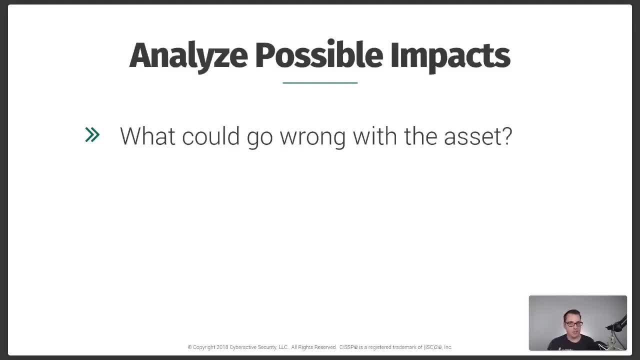 wrong. That is part of our job. availability, right. We need that server to be available when our customers want it. So what can go wrong? Those things have to get analyzed. What is the likelihood of something going wrong? What I mean? can it go wrong? Is it? 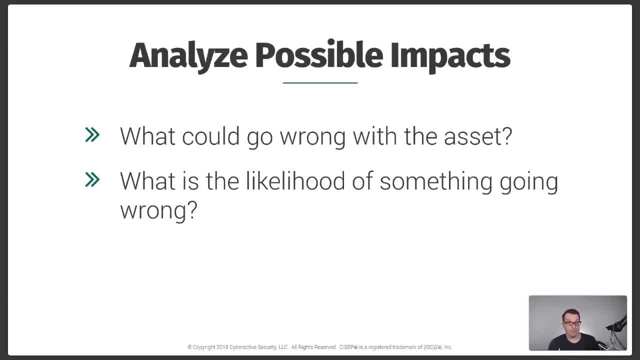 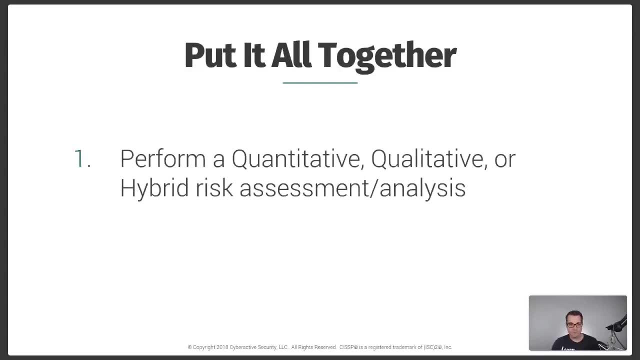 maybe likely. for sure I don't know, but we have to analyze those things And also what's the impact if something does go wrong. So when you put it all together, you're either going to perform a quantitative or qualitative assessment or you can do a hybrid. 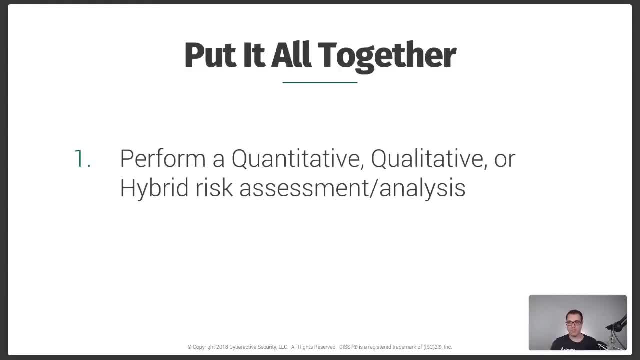 Most of us do hybrids. I like the quantitative because it's dollar amounts and that's what adds up to our managers. A lot of folks do qualitative because it's easier. It's a little bit simpler, right, And I'm going to walk through how to do each one of these just real quick. 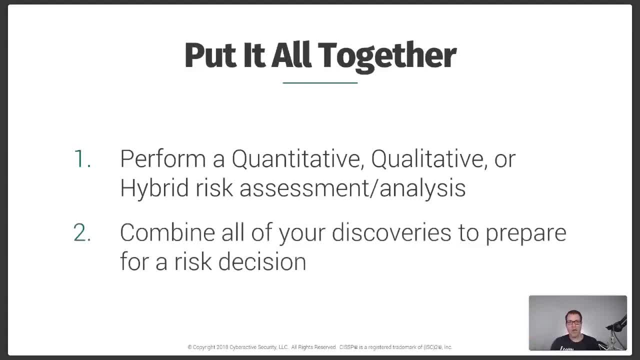 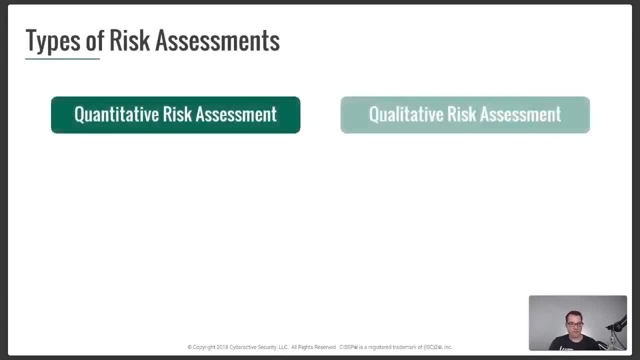 Um, and then what you're going to do is you're going to combine everything and then you're going to go ahead and and make a risk decision at that point. Okay, So this is how you actually do that. So you're going to have your 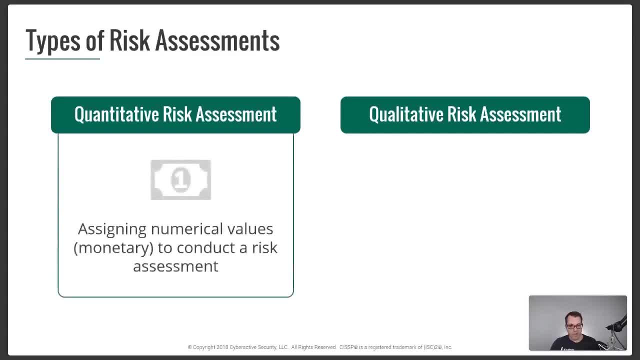 qualitative risk assessment, or your quantitative and your qualitative? The quantitative has to do with numerical values. Normally it's money. So we're looking at: how much does that web server cost? How much is it going to cost to replace? How long is it going to take to replace it? 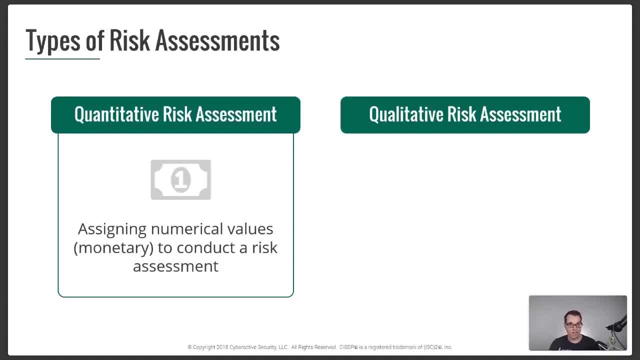 Meaning how long are we going to have to pay somebody to work on it, to replace it? How much does the software license is going to cost? If we have to replace something, all those different things come into play. Qualitative looks at things from a categorical 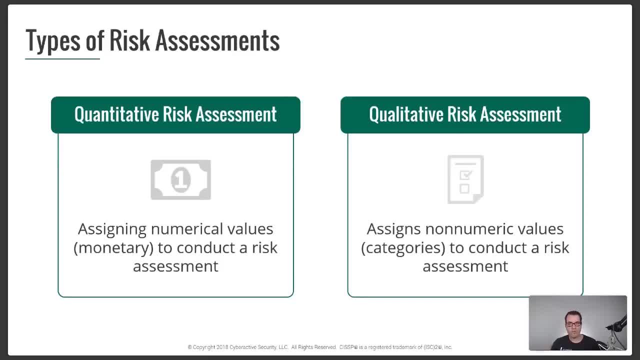 perspective: high, moderate, low, high, medium, low, whatever it is, Those are the two ways that you're going to do the risk assessment, Like, like I said, when you do the hybrid, you're combining the two. So maybe you're talking about how much a web server costs. 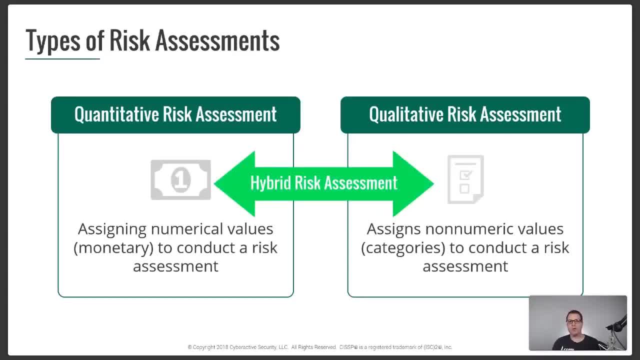 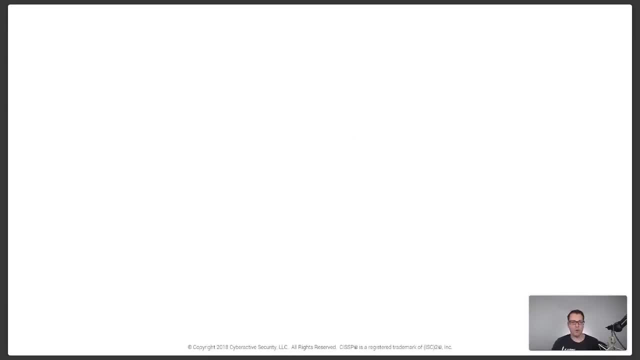 and what the labor costs are on it. But when you're talking about an exposure factor or a likelihood, you're looking at a high, moderate, low right. That's an easy way to think of it, So let me walk you through how this works. So we have these monetary and the numeric values, Like 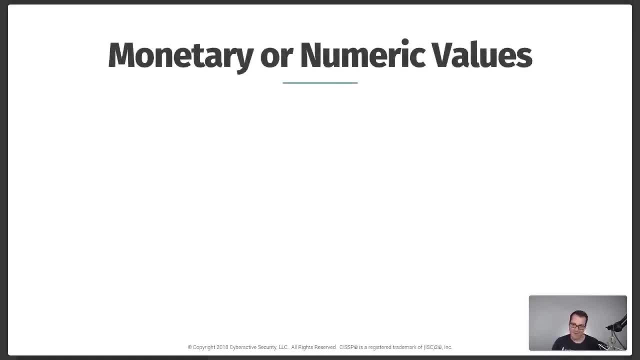 I said normally it's money, Cause that's what really really brings true with management and CEOs, right? So let's say this: this web server costs us 10 grand. right, That's pretty cheap. I mean, we just spent like 50 K on a on a server that we just bought was crazy, All right. So the 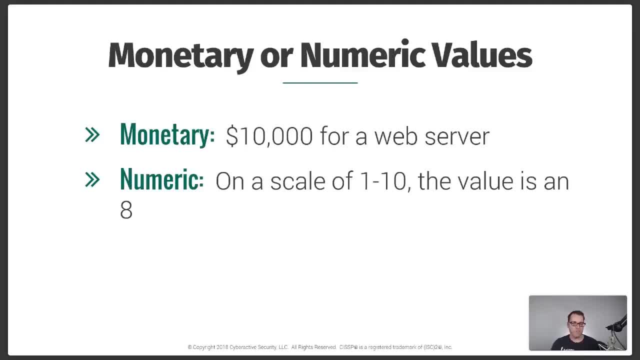 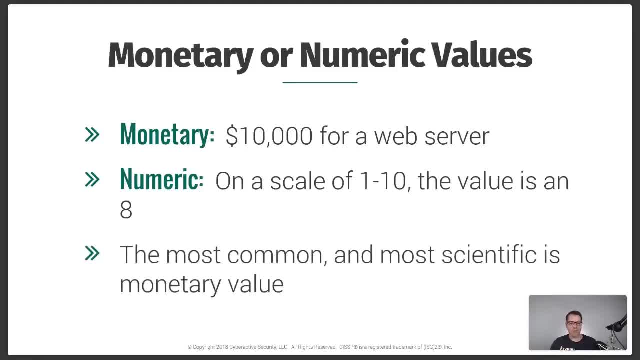 Okay, The most common and the most scientific way is to do the monetary value. That's how you really get down to the nuts and bolts. What's it really going to cost man? What's the real true impact? High, moderate, low is is really vague. but it's fast, It doesn't take a long. 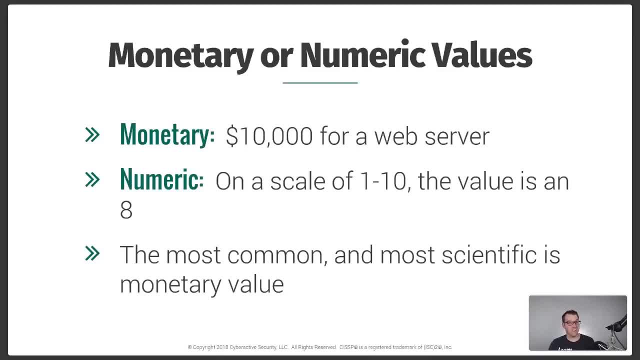 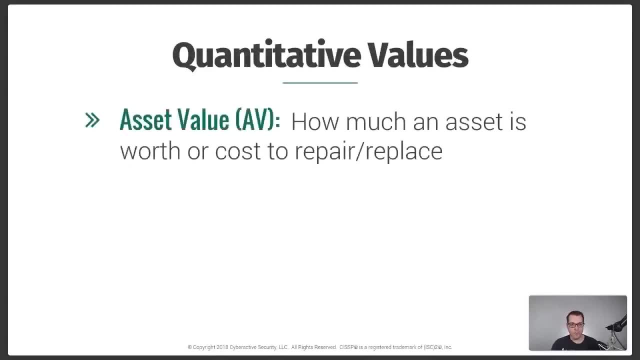 time to say: external facing web server, Yeah, Let's make that a high, real high, right. But if it's an internal web server, it's low. So it's pretty simple that way. So the way that we do the quantitative is: you're going to have your asset value, How much um is. 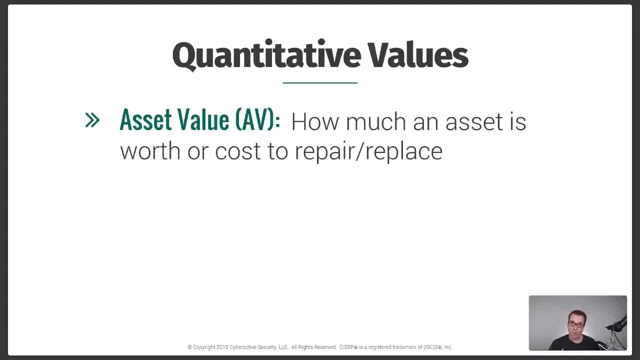 it going to be worth or cost to repair? And remember, we're talking to hardware, We're talking to software, We're talking to labor, all of the things that go involved. If that web server fails, what's it going to take to get it back up? And how much? how much of a check do I have to? 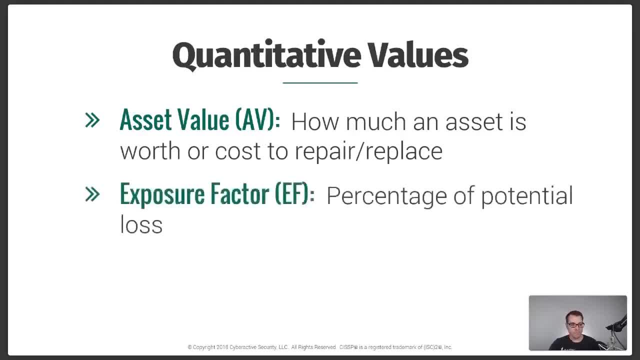 write to get that to happen. That's what we're talking about with our asset value exposure factor. What is the percentage of potential loss? So, if the web server was to be DDoS, how much of that web server is going to be compromised? How much of it's going to be? 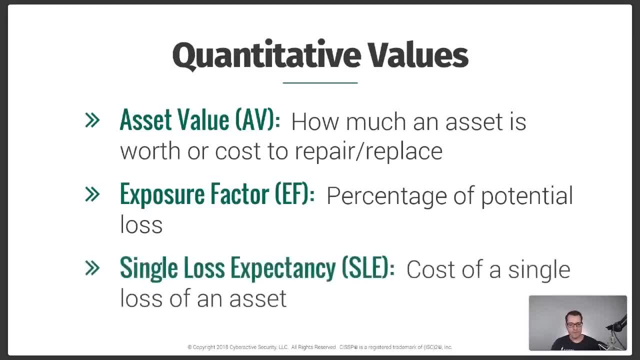 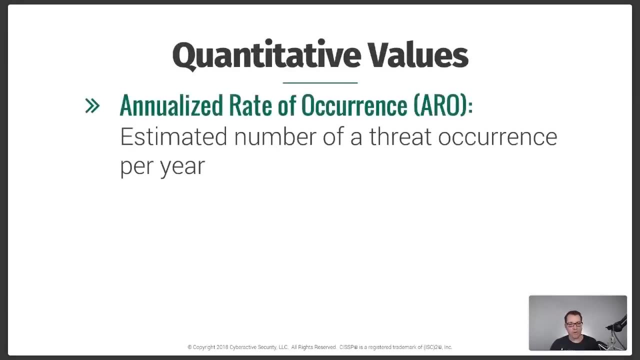 impacted and destroyed. Okay, Single loss expectancy. This is a cost of a single loss of an asset. So if the web server got attacked one time, how much do we expect to lose in that process? And then we have: um, we have our annualized rate of occurrence. So this is the 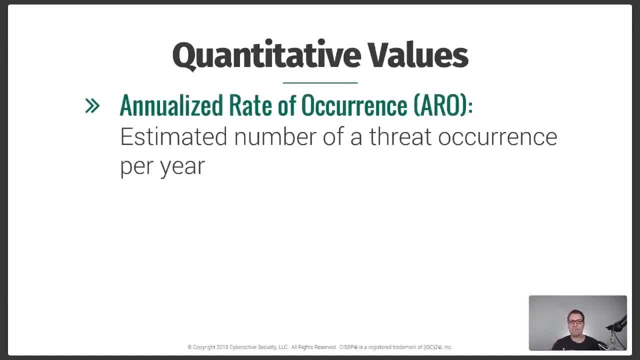 estimated number of threat occurrences per year. So how many times do we expect this to happen to the web server? And then we have our annualized lost expectancy and that's the annualized cost overall for the year. So we have our single loss, our SLE single loss expectancy. That's how. 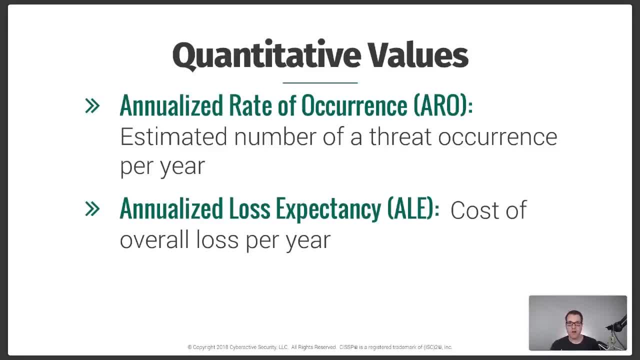 much it costs for one time. How many times is that going to happen? That's our ARO And then your ALE is the combined total of that. Okay, Let me show you how all that works. Oh, and then we've got the safeguard. Forgot about that. Annualized cost of safeguard ACS. 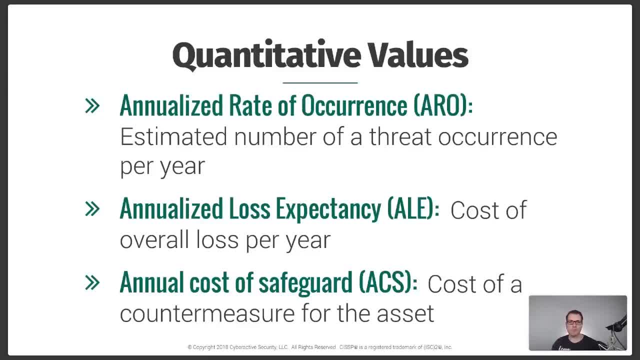 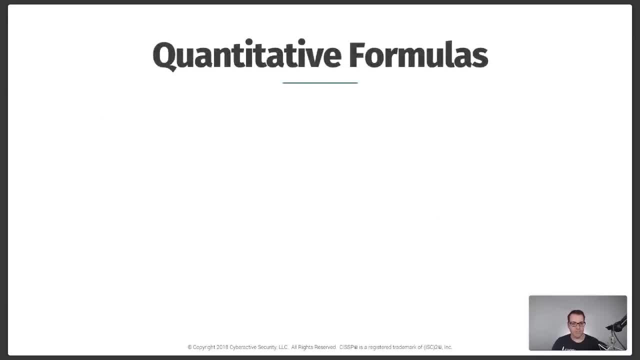 This is what you're going to put in as a countermeasure, and how much you have to spend on a countermeasure to protect whatever it is, in this case, the web server. Okay, So I was wanting to jump to this slide right here. Okay, So this is how it kind of works. 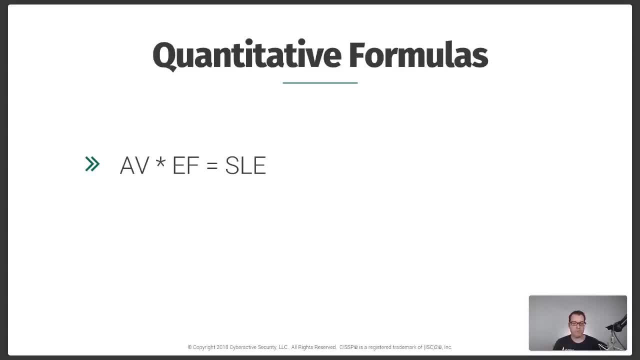 You're going to take your asset value and your exposure factor, You're going to multiply those and that gives you your, your single loss expectancy. So, again, I'm going to show you how to do this in your head. I'm going to give you a perfect example of how to do this. 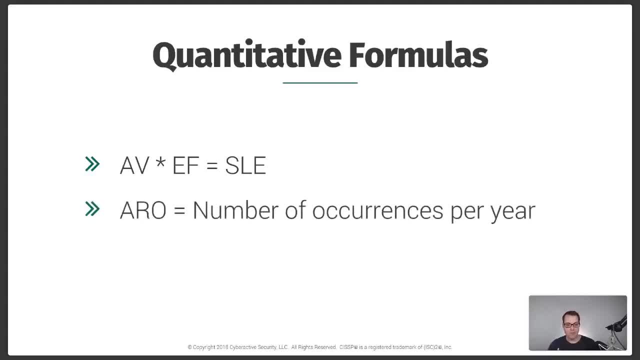 The annualized rate of occurrence- ARO. that's the number of times it's going to happen throughout the year. And then we have the SLE times. the ARO It's going to give you your ALE. So let's take a look. 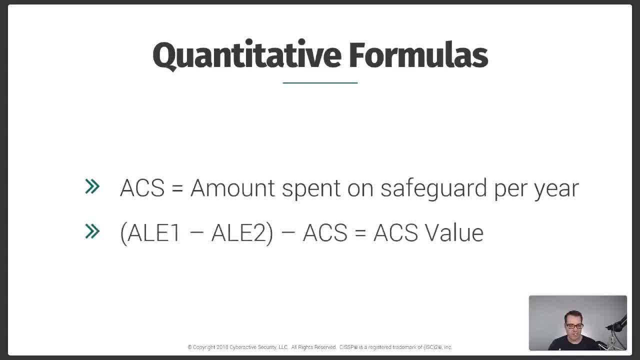 And then you have your ACS right, Which is how much you're going to spend on the safeguard. Normally, what you're going to do with that is you're going to take two annualized loss expectancies and you're going to measure the difference. So you're going to look at one. 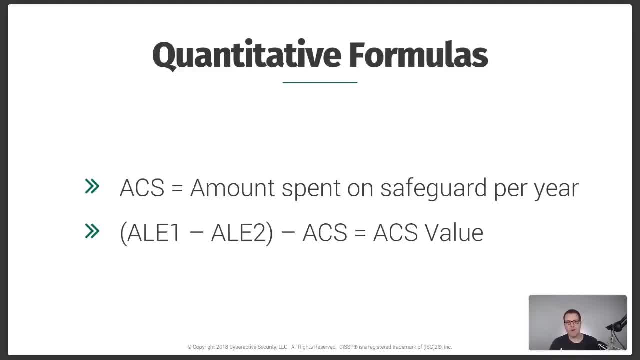 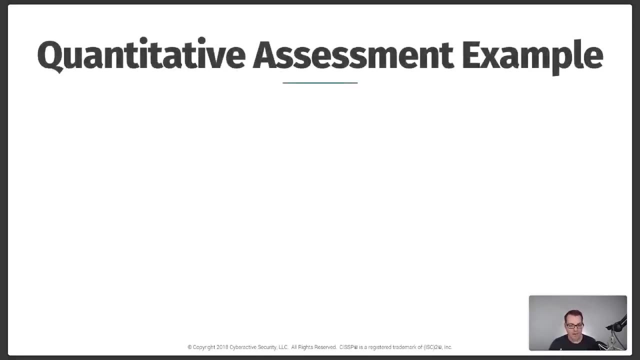 let's say, um annualized loss expectancy is 8,000 bucks for that web server. And then when you apply the countermeasure- firewall and point security, whatever it is you do now, it reduces it to 4%, $4,000.. That's your ACS value. Okay, I'm wanting to get to the slide, because I know it's right here. 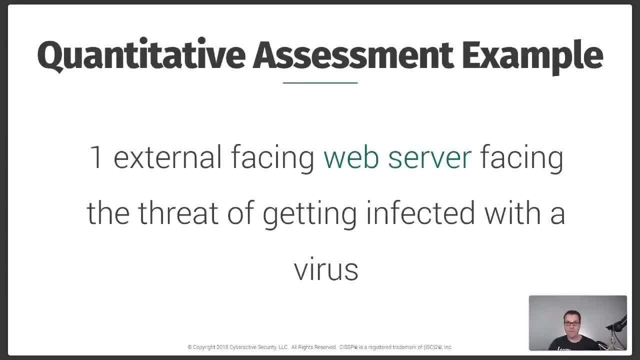 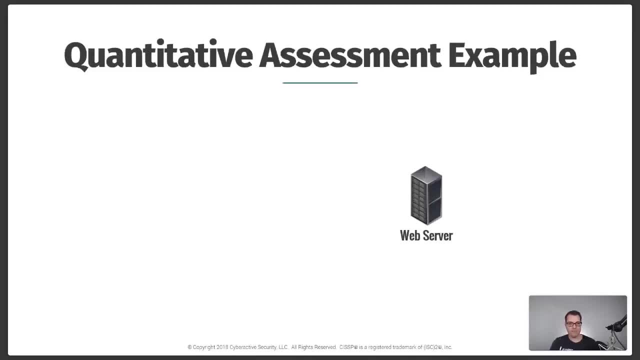 There, it is All right. So that one external face facing web server that we talked about before, it's the same run. Okay, So here we go. You have your web server sitting out there on the internet waiting to get picked off. I don't know why I went with that. So let's say that this thing costs 10. 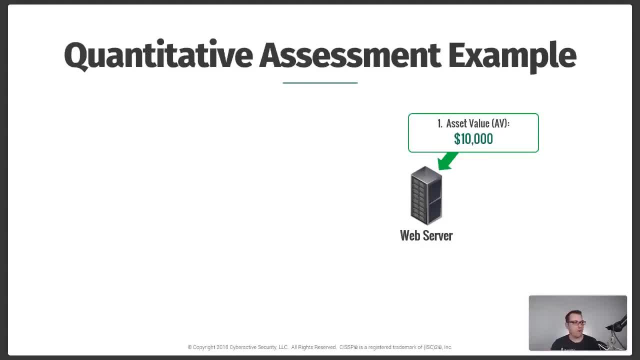 grand. Okay, Um, like I said, we just bought a server, Uh, we just bought an app server, uh, at work, and we spent 50 K on it, Um, and then we're going to go to the next one. So let's say that this thing costs 10 grand. 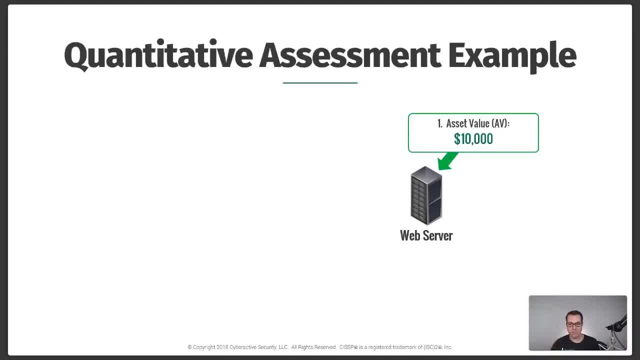 I mean it's it's. uh, it was designed to be a hypervisor, So anyway it's it's loaded man, I mean the things I'd love to have it at the house should probably steal it from work. 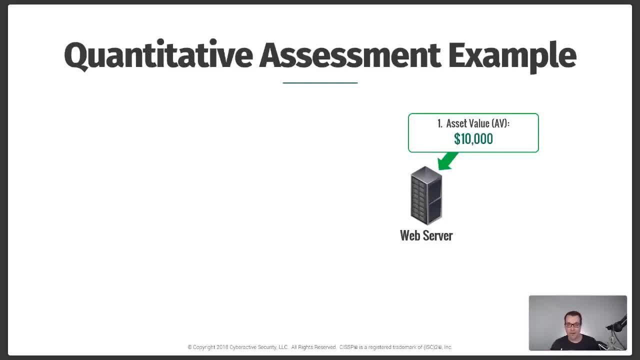 Don't tell anybody I said that. So anyway, you have the web server. that's 10 grand. That's a little cheap, but it's 10 grand. So remember that the asset value has to do with the hardware, the software, the labor, the maintenance, patching, upgrades, all the things. 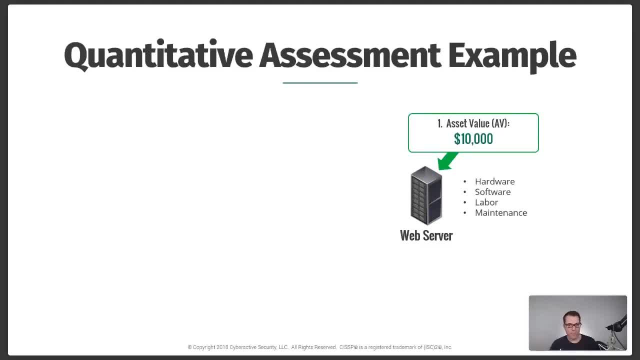 that we have to do to it, Right? So, um, if we have to upgrade memory cause it's too slow, or if we have to add a new hard drive cause we run out of space, or whatever the case is, we want to add all of that in there. So let's say everything, total is 10,000. 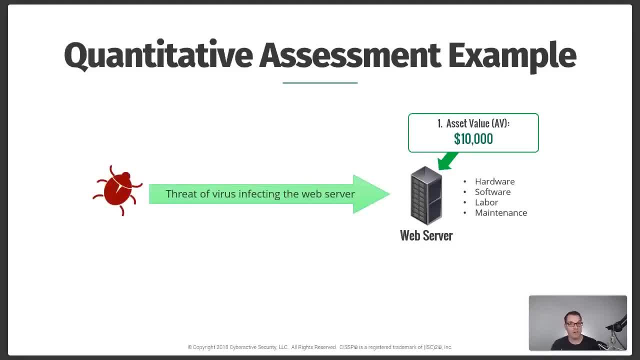 And then we got our little critter right That's going to come out and try to attack this web server. Okay, So that's your threat And the exposure factor is, let's say, you get a virus on the server. If you get a virus on the server, we're expecting to lose about 80% of that server. 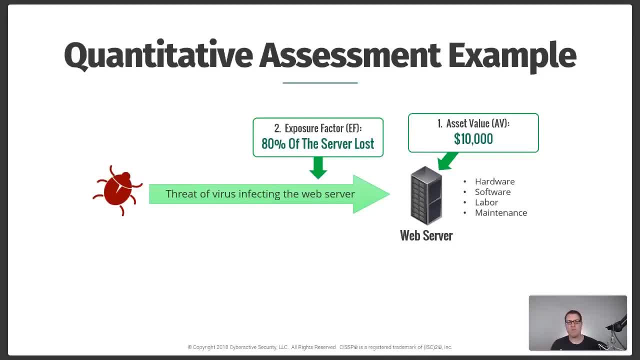 That means we have to rebuild 80% of that server, whether it be you know. uh, obviously most viruses are not going to damage the hardware per se. I mean, there are ones out there that can do it, but by today's standard that doesn't happen as often. 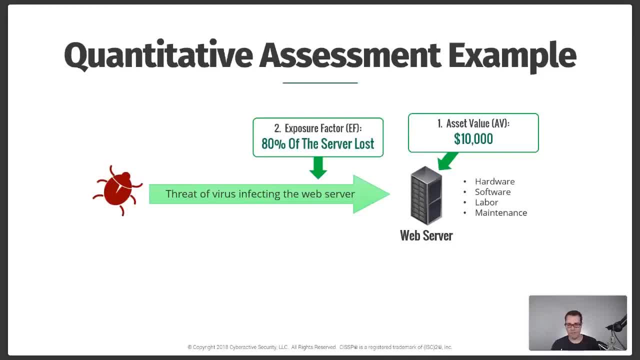 as you would think it does. Um, mostly the software apps are what's targeted. I mean, it's just the easy pickings. So, um, you're not going to have any maintenance on it at that point, cause it's down, So you're going to lose about 80% of it. That's what we're expecting here. 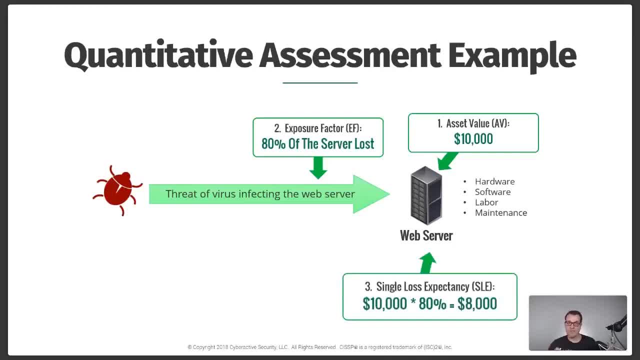 Then your single loss expectancy is that 10,000 times 80%, which means it's 8,000.. So every time we get a virus on the web server, we're expecting to lose $8,000.. Is this making sense? Okay, I know that's a lot of numbers and a lot of math. So 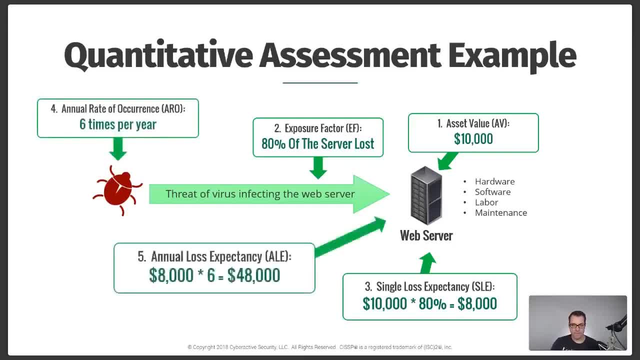 gosh, keep going. There you go. And let's say, our annualized rate of occurrence is we expect this to happen six times throughout the year, Then what we're going to do is take that 8,000 from the SLE. 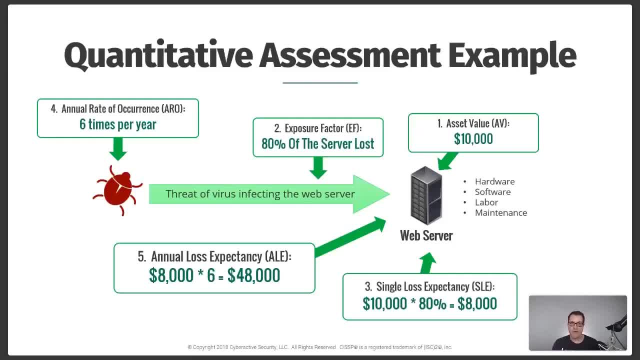 We're going to multiply that by six times and that's $48,000.. So that means we need to stuff $50,000 away somewhere to protect that web server, to be ready for it to crash, be ready for it to be attacked, to have a virus hit it, whatever the case is. 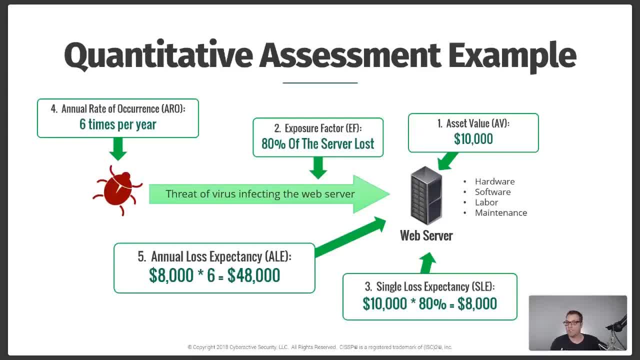 We need 50 grand to make sure that that web server is going to stay up and running for us at all times. Okay, That's how fast you can do this. 10 grand, What do you expect to happen? The exposure factor is just a guess. I mean there's no way to really quantify. 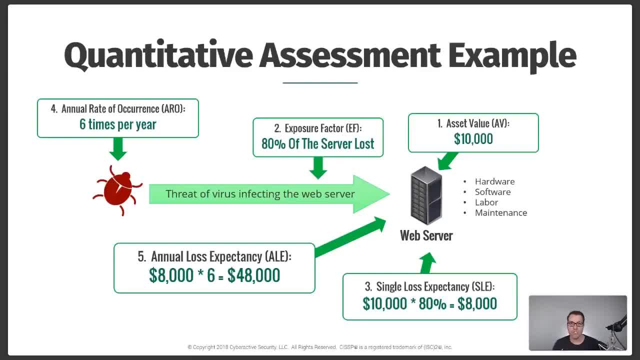 how much you could lose, because it just depends on the virus, right? So we just assume, we just, yeah, Probably 80%, man, We're going to have to reinstall the web OS, We're going to have to have somebody work on it, blah, blah, blah. Yeah, It's going to cost you about eight grand. 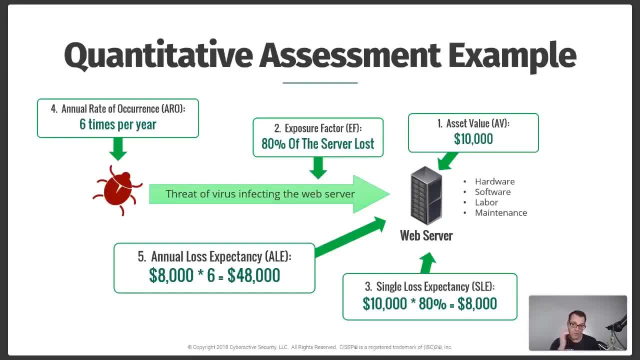 every time it happens? Very easy. How many times do you think this happens? Well, judging by the traffic we see, it's about four or five times a year. So let's say, six Done Bam Need 50,000.. Now you can go back to the boss and say, hey, 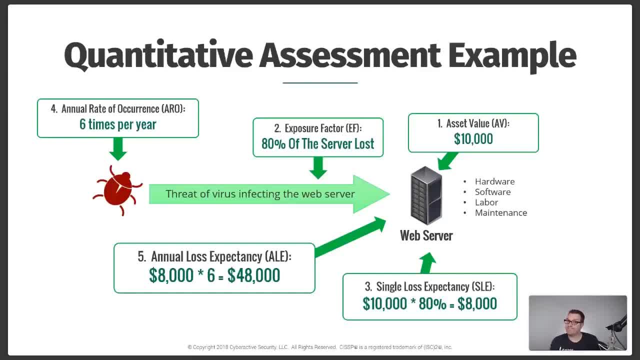 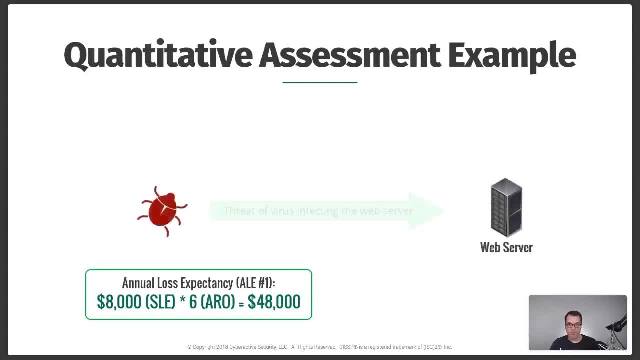 we need 50 grand to cover this server. Okay, Now the option is you have your 48,000.. That's your ALE. So you just have your web server again and you got your little critter who's going to attack. 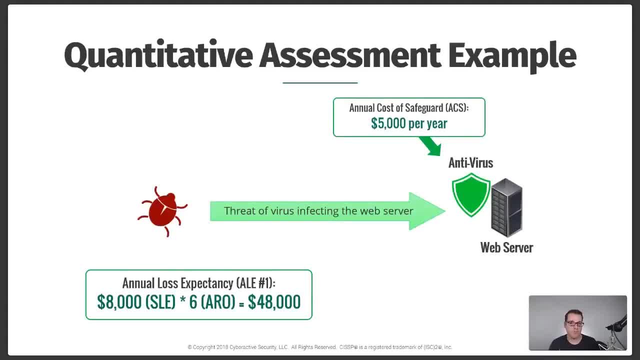 Now let's say we install an antivirus on there, anti-malware software on the web server, And that costs us five grand a year, right, Because we went with Symantec or McAfee. They're pretty pricey, right? So if you do McAfee, EPO, the APO e-policy orchestrator and you deploy all their little, 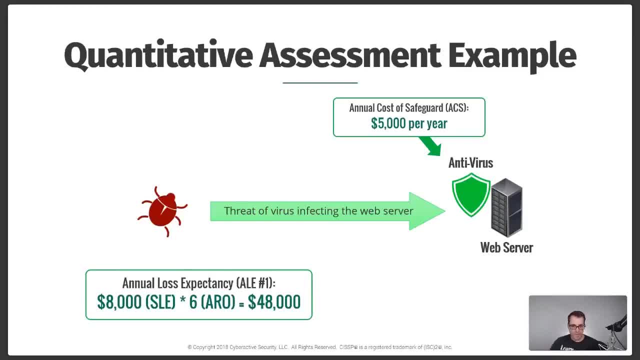 stuff. yeah, it'll run you five grand a year, easy. So you install that on there and that's going to cost you 5,000 bucks. But we're going to determine that now that we have protection, maybe we're only going to get. 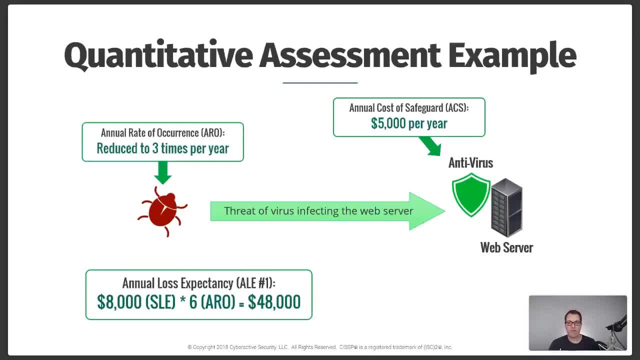 we're going to see three of those six attacks become effective. The other three will get blocked because McAfee's okay, It's not great, It's not the best, but it's pretty good. So it will reduce the attack to three versus six. So now, what you're going to excuse me, what you're going to do. 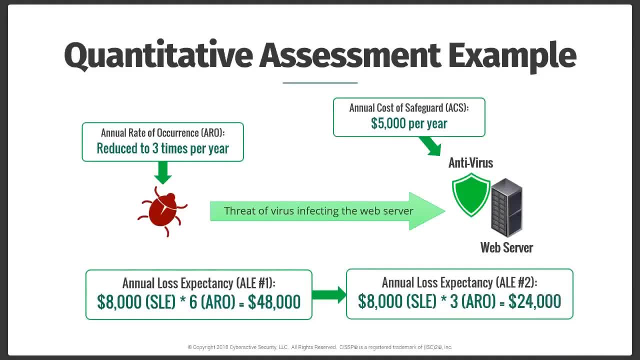 is you're going to calculate- and my mug is right there, So let me, there we go. So now you can see um. so now you're going to take the first annualized loss expectancy, 48,000, and then 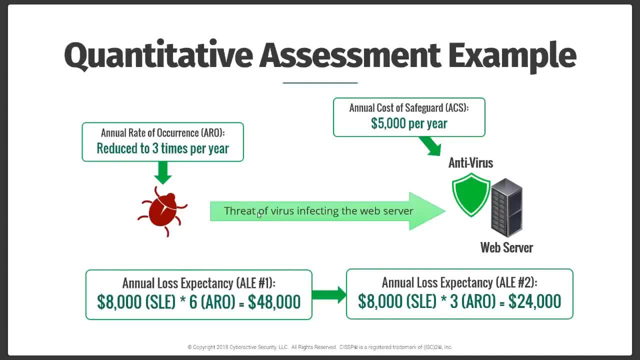 you're going to subtract the um, the other ALE for 24,000.. So you're looking at 8,000 times three times this time. So now you basically just cut it in half. So now your ACS value is what you're. 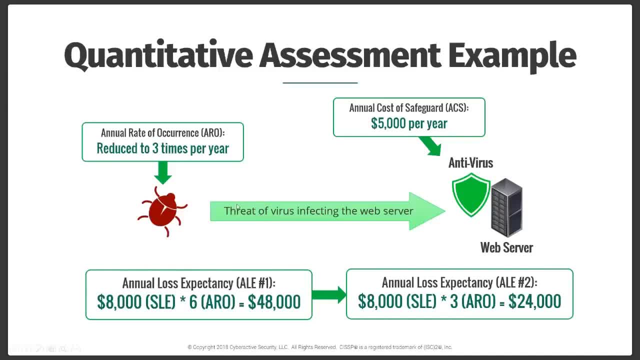 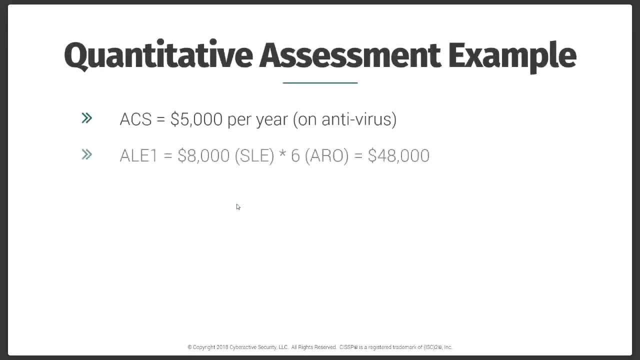 trying to get here And my slides aren't moving. There we go. So the ACS is 5,000 per year. right, We're going to take the first ALE: 8,000.. We're going to multiply that by. 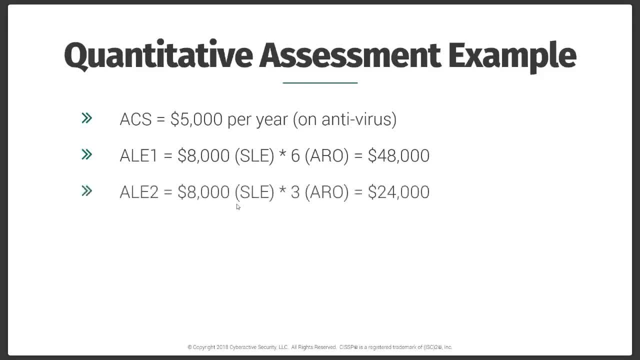 the six. that was without protection in place. The second ALE is with protection in place and we're cutting that in half. So we're saving $24,000 just by deploying McAfee- EPO McAfee, You owe me an affiliate check. I just made you some money right And now you take your. 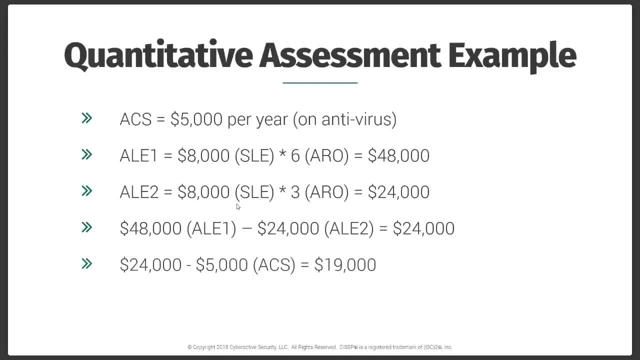 annualized loss expectancy minus the amount of money you're spending on the countermeasure, And you just saved 19 grand. So now you get to go into the boss's office saying: Hey man, I just saved you 19,000 bucks. Pretty awesome, right? That's how. that's how fast you do this. 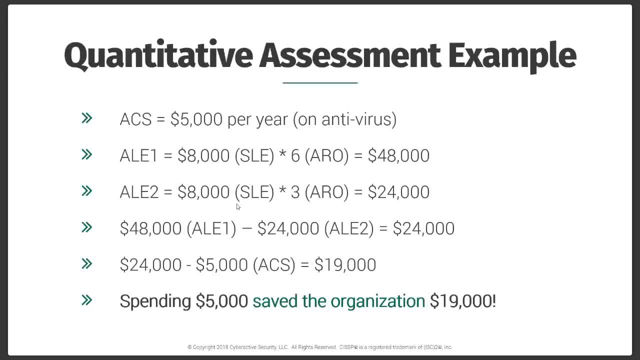 And what's funny is, even though people don't- people use all these fancy tools and all these fancy things. they do not think about things at this level. Now, this is obviously a very like complex, you know, calculation of stuff, but I do this in my head. I'm not this accurate. 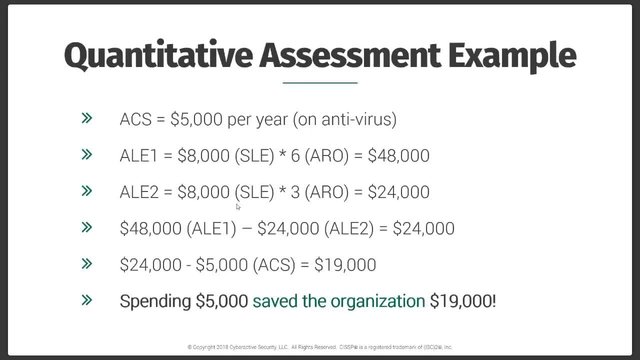 but I'm pretty and close, like what's the web server costs this? Well, how many you know how long do we have to work to to get this up? about two hours Okay. So we're paying some dude like 50 bucks an hour. 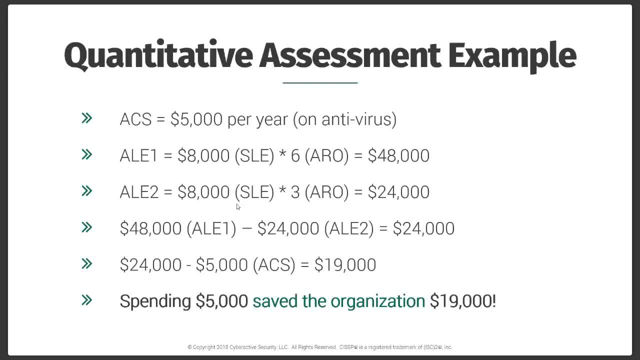 Okay, So that's you know, a hundred bucks, you know, on his end, blah, blah, blah, blah. Okay, Yeah, Let's do this and let's deploy that. done, You know, that's. I mean, that's the level I. 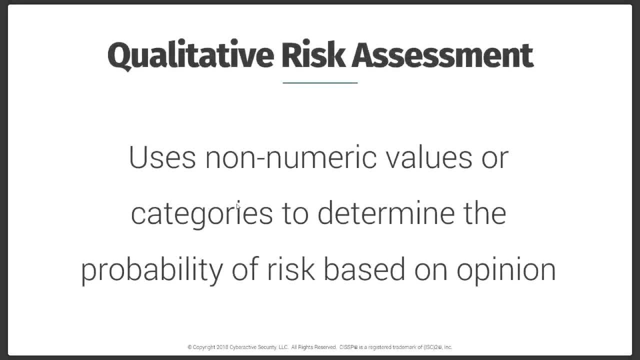 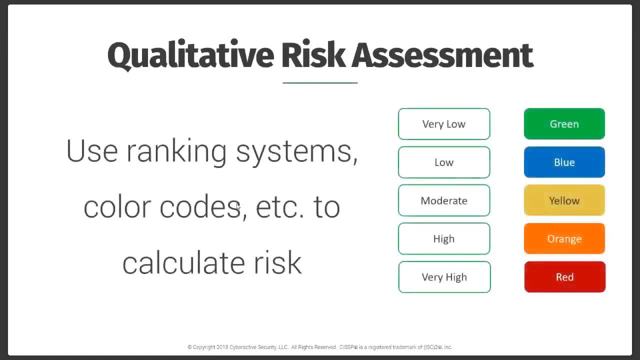 think on it anyway. Okay. So when you're putting this all together, you know that's the monetary side of the house. Now you're actually going to just look at the categories. So, using that same exact example, right, We're going to use, instead of numbers, we're just going to use- green, blue. 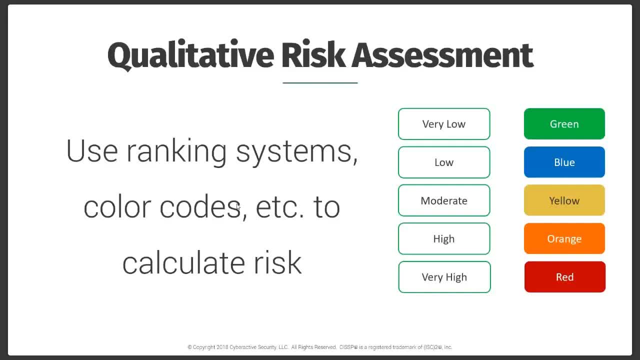 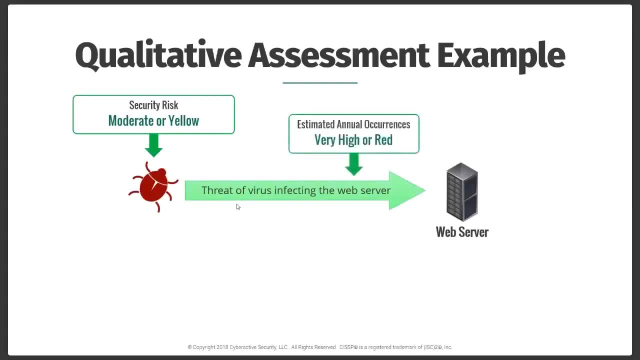 yellow, orange, or we're going to do low, low, moderate, high, whatever the case is Okay. So we had that same setup. You have your threat, you have your your, you know your web server and the security risk. Maybe we just see it as a moderate or a yellow and the rate of occurrence. 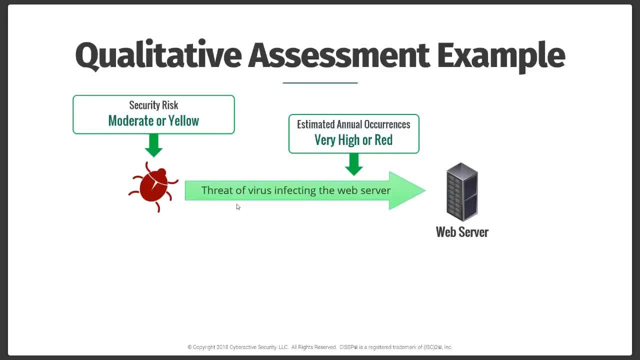 Yeah, It's probably going to be a very high or red, because it's going to happen a lot. right, External facing server: Okay To replace it, And it's pretty low considering I mean 10 grand for a server and a fortune 500. 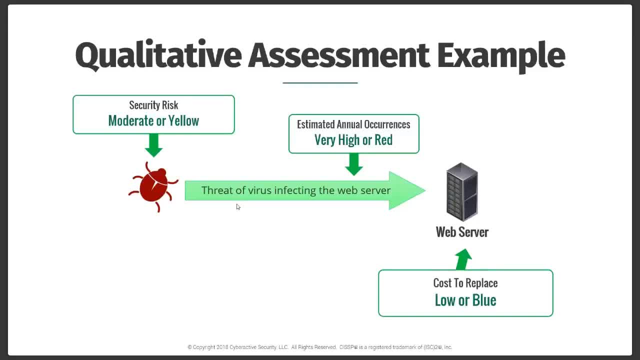 company, that's a drop in the bucket, man, But if you're a small business, that's a lot of money. So, again, that's why the risk assessment is so important, because not everyone is the same and the risks and the threats to everyone's system is not the same. Everyone has unique data. 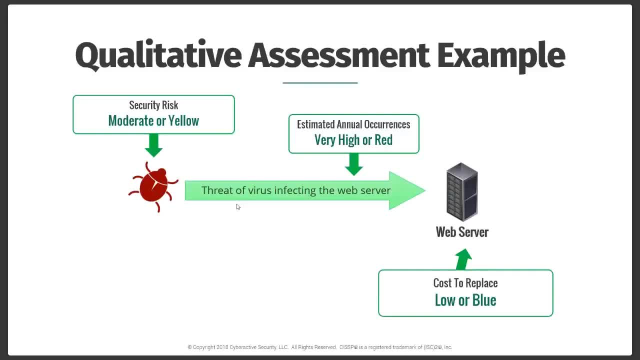 unique systems, unique things. So in our case, maybe in a fortune 500 company, yeah, it's low. whatever man, 10 grand to freaking write off, We'll do that. But if you're just running a, a small shop, 10 grand for a server is a lot of money, right? So at this point,